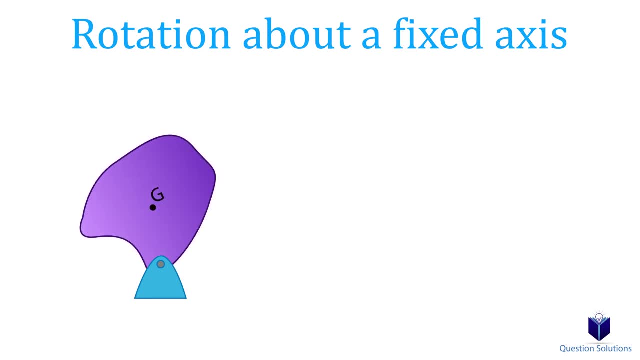 object that's rotating about a fixed axis. That means angular velocity is not zero. In that case we can find the kinetic energy by using this equation. We have the kinetic energy when an object is translating, plus we have a new part, which is the mass moment of inertia about the. 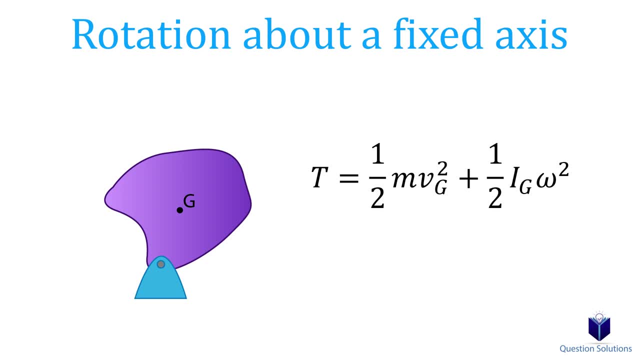 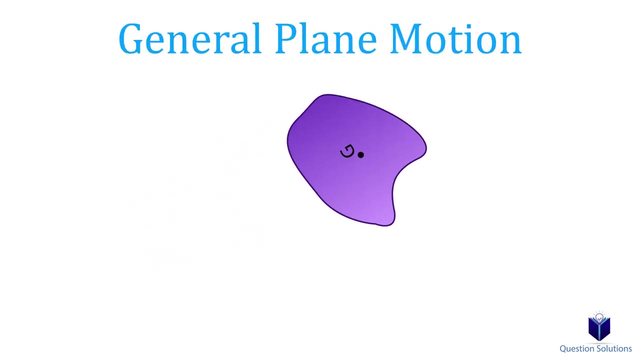 center of mass times the angular velocity squared. If, however, instead of using the mass moment of inertia for the center of mass, we find it about another point, for example point O, then the equation becomes this: Lastly, we have the general plane motion of a rigid body. In that case, we use 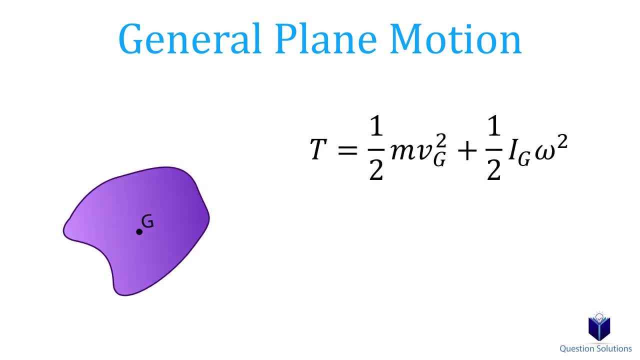 the same equation as before and use the mass moment of inertia about the center of mass. If you go through the steps to find the instantaneous center of velocity, you can actually write this equation in a simpler form like this: In this case we are finding the 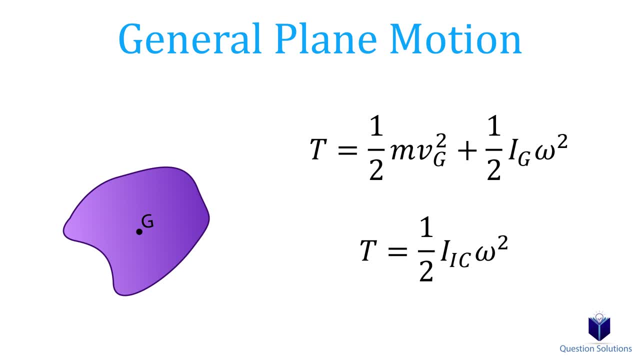 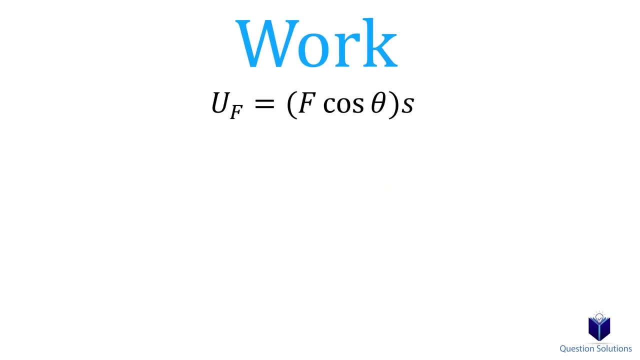 mass moment of inertia about the icy point. Now that we know how to find kinetic energy, let's talk about work. Work is basically force times distance, and I cover this in detail in the kinematics video about work and energy. So I will glance over the stuff we need for rigid bodies. 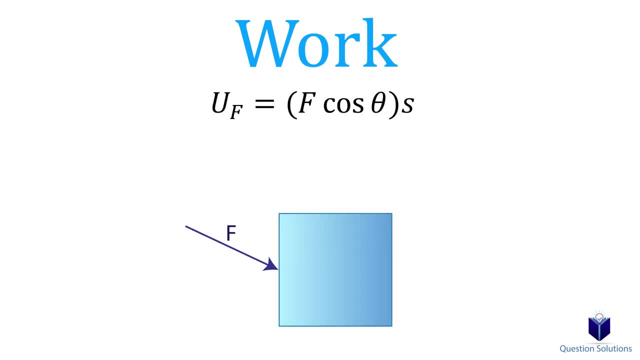 Let's say we have an object like this and we apply a force at an angle, The work that's done is force times cosine, theta times the distance traveled. This is when the force is a constant. If it's a variable force, we can integrate it like this to find the work done. 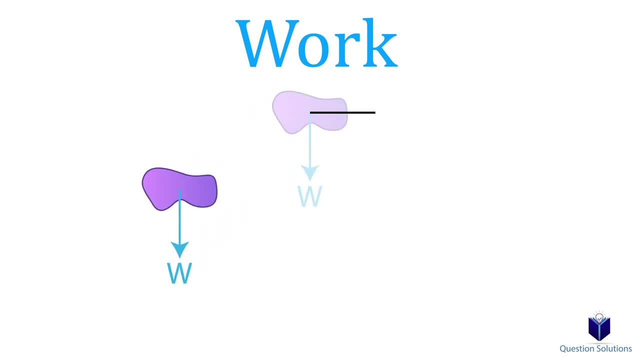 When we consider an object that's moving up or down and think about the work that's being done by the weight of the object. we can figure it out using this equation: Delta y is the vertical displacement. If the object moves downwards, it's positive work. 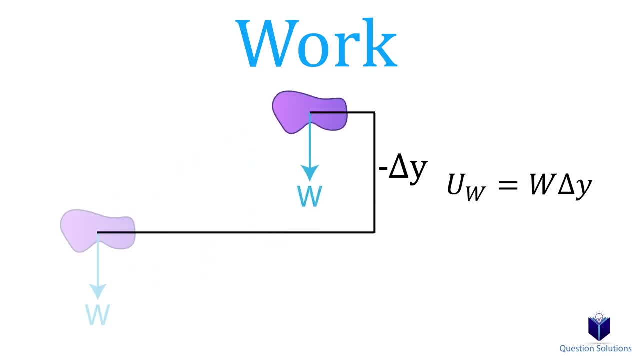 and if it moves upwards it's negative work. This is because weight is opposite to the displacement. Next, we got the work done by springs. If we have an object attached to a spring like this and we pull it to the right, the spring will create a force where it's trying to bring the 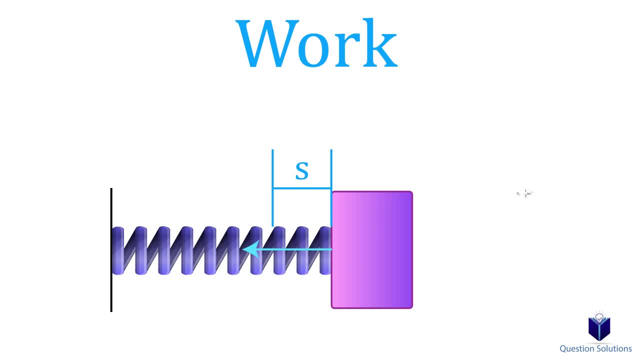 object towards the left. The work that's done by the spring can be found using this equation: S is the elongation or compression of the spring and k is the stiffness of the spring. The last factor we need to consider is work done by a couple of moment, If the moment is not constant. 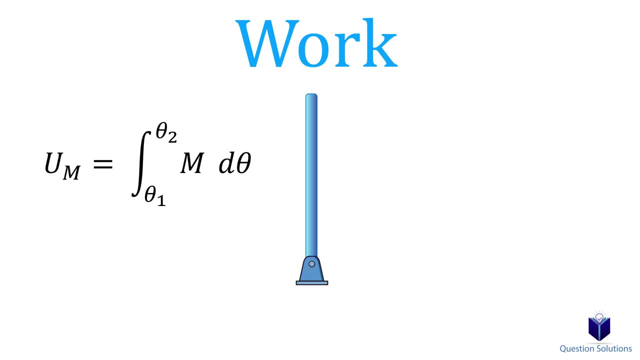 we can figure out the work done by this equation. The initial and final theta values are in radians. So if we have an object like this and due to a moment, it's spun 90 degrees, then the lower bound would be 0, and the upper bound would be pi over 2,. 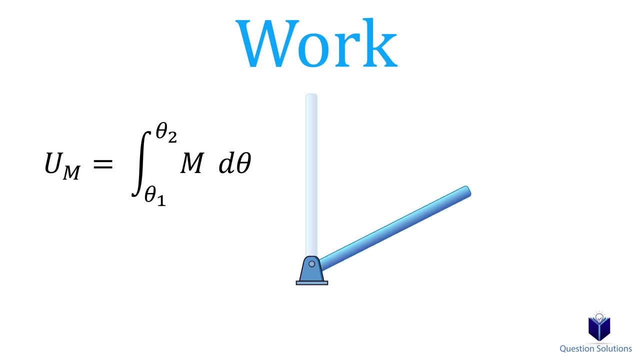 since that's 90 degrees in radians. If the moment is a constant, then we can figure out the work being done by this equation. You should also note that some forces will do no work. For example, if we have an object pinned like this, the reactions at the pin won't do any. 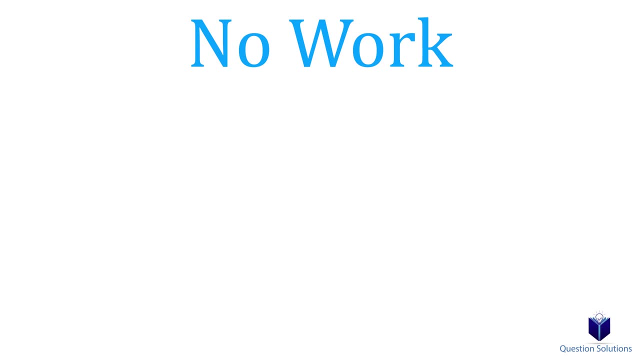 work since the pin is fixed. Another example would be when something rolls along the floor but isn't organize. If it doesn't slip, the friction does no work And, of course, if the force is perpendicular to the displacement, it does no. 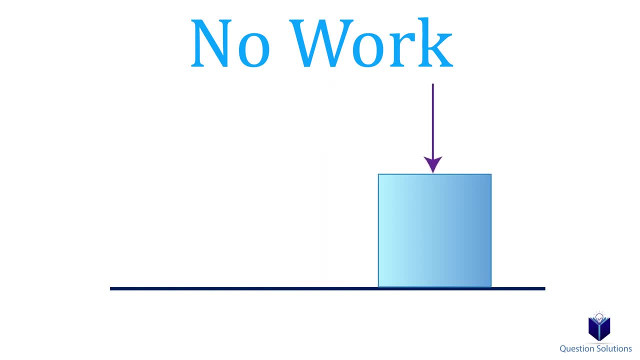 work. In other words, let's say an object moves only in the horizontal direction, then vertical forces will do no work, since the object doesn't move up or down. So again, a force only does work when it moves through a displacement in the direction of the force. 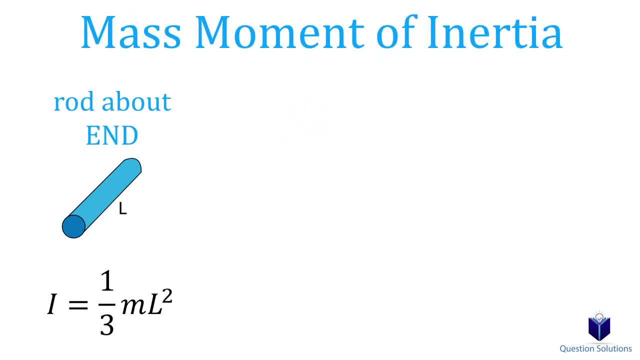 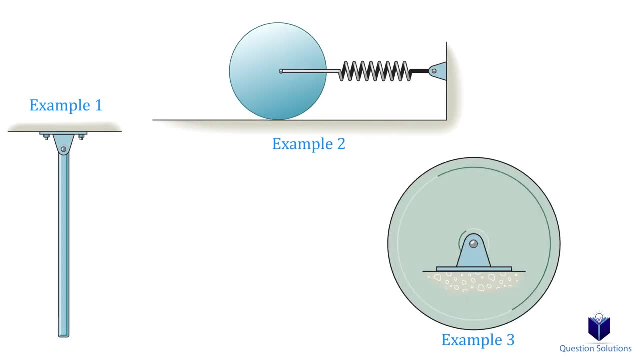 For some questions. you need to figure out the mass moment of inertia for objects. I show some formulas here, but you can find many more online by searching for them. Now let's get started with some examples to see how and when to apply the equations we talked about. 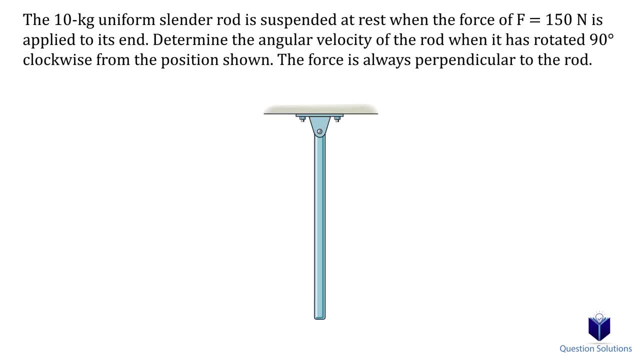 Let's take a look at this problem where we have a rod at rest. Then a force of 150 newtons is applied to the bottom of the rod and we need to calculate the angular velocity when it rotated 90 degrees. Let's draw a free body diagram of the rod. We have the reactions at pin O. 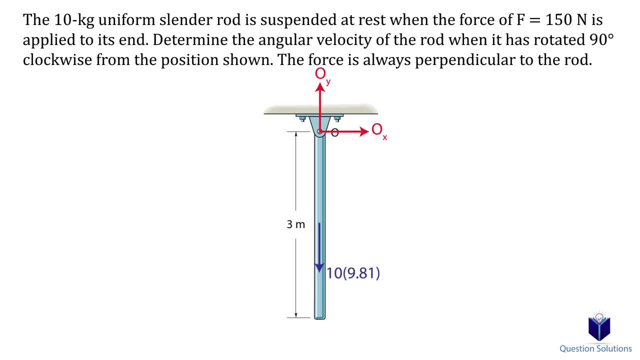 so this is a rotation about a fixed axis. We also have the weight of the rod at the center, and let's not forget about the 150 newton force applied at the bottom. To solve this problem, we're going to use the principle of work and energy. Let's write down the equation. 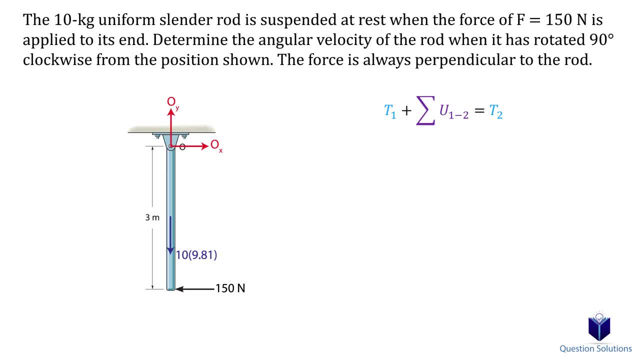 We will do each segment separately and then plug everything in. So first we need to think about the initial kinetic energy. The whole system starts with the initial kinetic energy. For the final kinetic energy, since this is a rotation about a fixed axis. 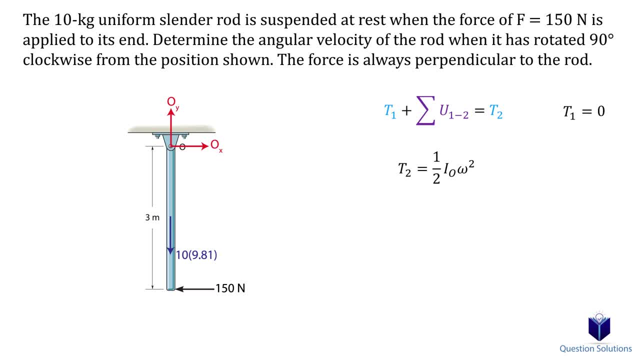 we can use this equation, But to use it we need to figure out the mass moment of inertia for this rod at point O. So for that, the equation is this: It lets us calculate the mass moment of inertia at the end of a rod. Since point O is at the end, we can use this equation. 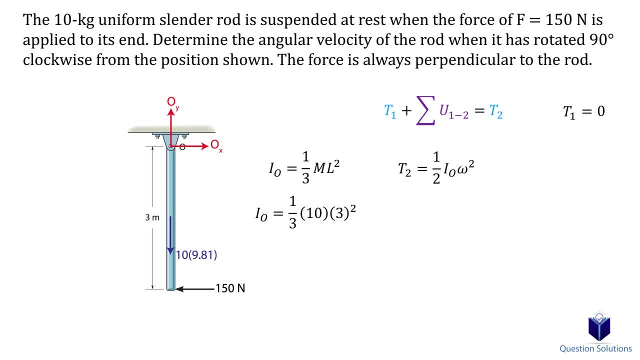 So we have a mass of 10 kilograms and a length of 3 meters. Let's solve, Let's plug in the mass moment of inertia we found into our kinetic equation and set it aside. Now we have to consider work. The work is done by two forces: the weight and the 150 newton force. 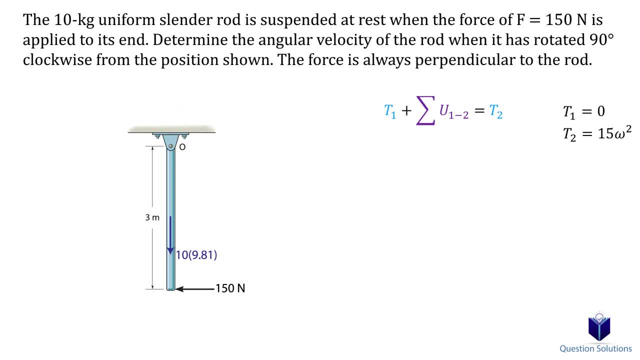 The reaction at pin O does no work since they don't move. The two forces that do work are both constant, so we don't need to integrate First. we will focus on the 150 newton force, which does positive work since it's pushing the rod where we want it to go, which is clockwise. So remember: 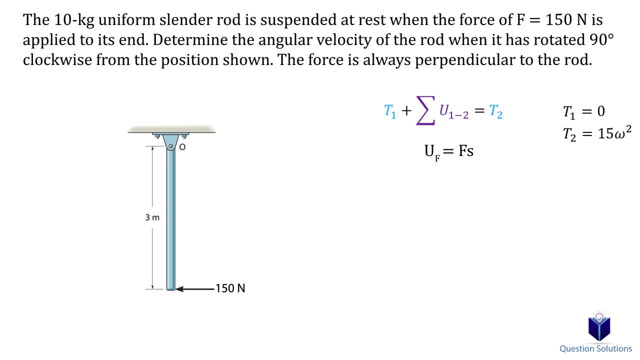 work done by a constant force is force times distance. So what we need is the distance for which the 150 newtons acted on the rod. We know that the rod turns 90 degrees and in radians that's pi over 2. And we can find the distance by multiplying that by the length of the rod. 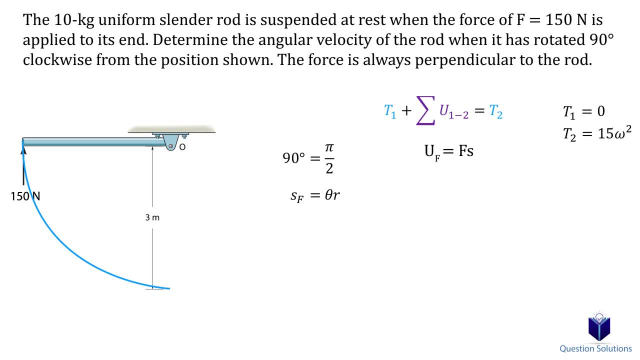 Or rather think of it as the radius, Think of the end of the rod drawing a circle. so it's just the arc length we're trying to find. Now we can figure out the work done by the 150 newton force. Next is the work done by the weight. 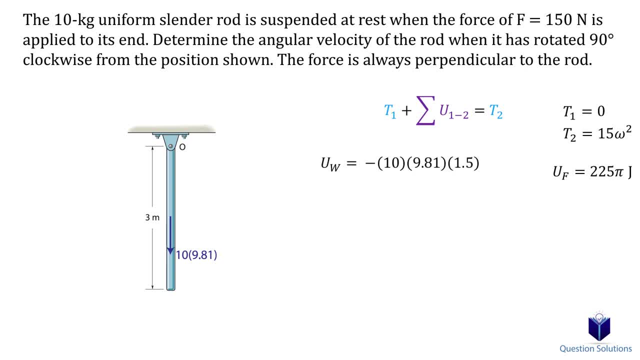 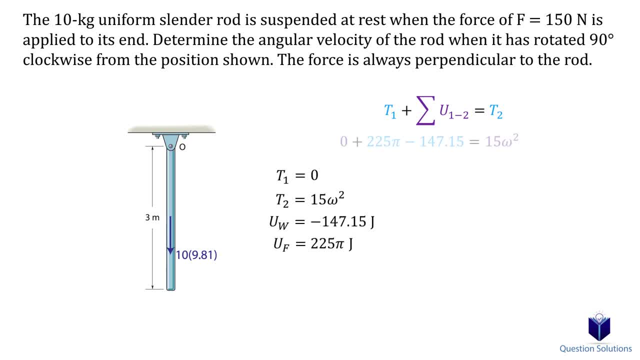 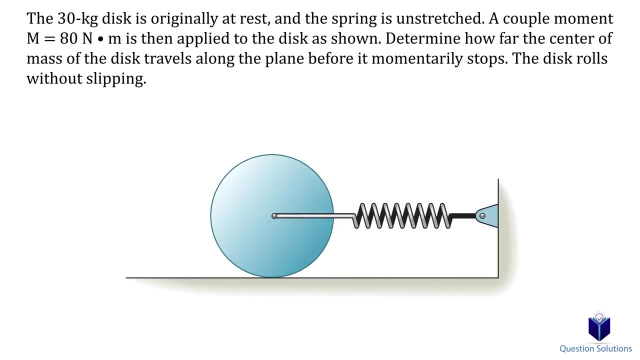 meters. Now all that's left is to plug in the values. Let's solve for the angular velocity, and that's our answer. Let's take a look at this problem where we have a disc attached to a spring. Then a couple moment is applied to the wheel and we need to figure out how far the center of the 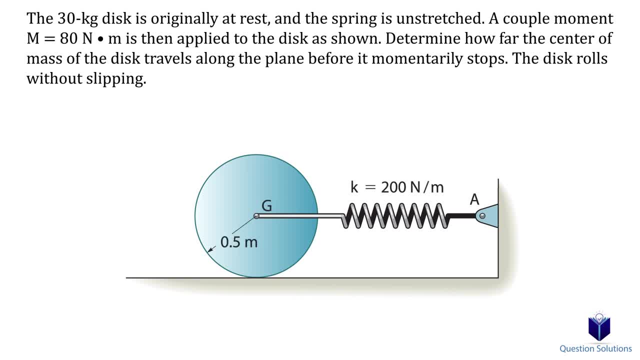 wheel will travel. before stopping, Let's draw our free body diagram. We have the weight, the force, spring, the moment and the normal force, Since the disc rolls without slipping. we don't need to worry about friction for this question, because it does no work. 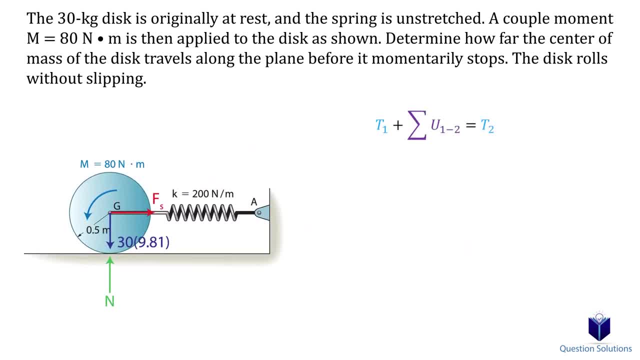 Now let's write our principle of work and energy equation For the initial and final kinetic energies. they will both be zero, since the disc starts from rest and stops at the end. Now two forces will do work, which is the spring force and the moment applied to the disc. 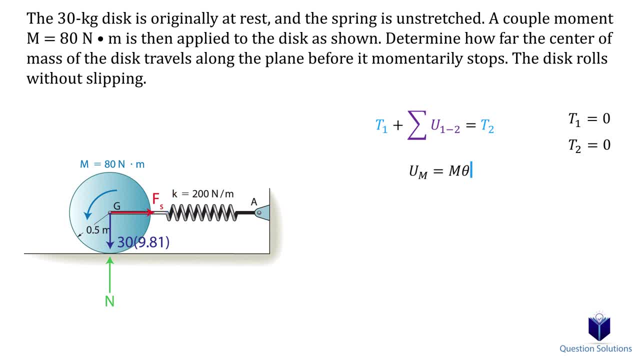 To figure out the work done by the moment, we need to figure out the theta value or, in simple terms, how much the disc will turn, Since, as before, this is arc length. we can write our distance like this. Let's isolate it for theta after we plug in the radius, which is 0.5 meters. 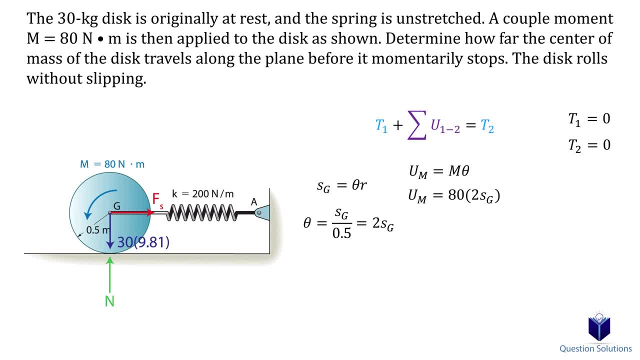 Now we can figure out the work done by the moment. We know the moment from the question and we wrote the theta value in terms of the distance moved. Let's simplify Now for the work done by the spring, Since the spring is trying to stop the wheel from. 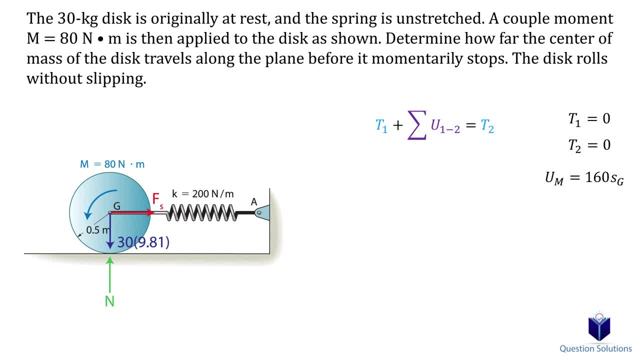 going forward. it does negative work. Let's write the formula for work done by a spring: The stiffness is given to us and the distance it stretches is the length the wheel travels. All that's left for us to do is plug in all of these values into our work and energy equation. 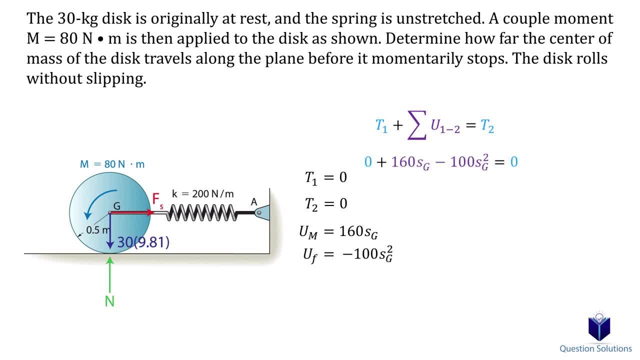 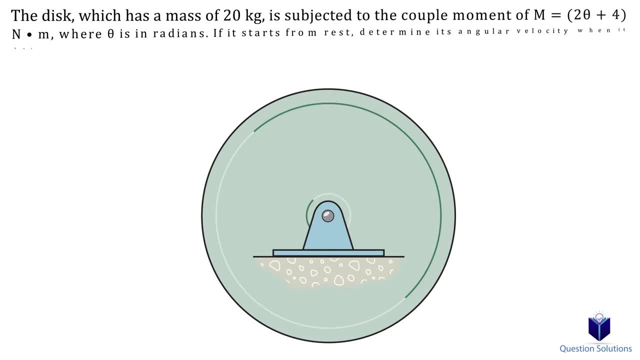 Solving this equation will give us two values: 0 and 1.6 meters. It's definitely not 0 meters, so the answer is 1.6 meters. Let's take a look at one last question, where the moment applied is not a constant. 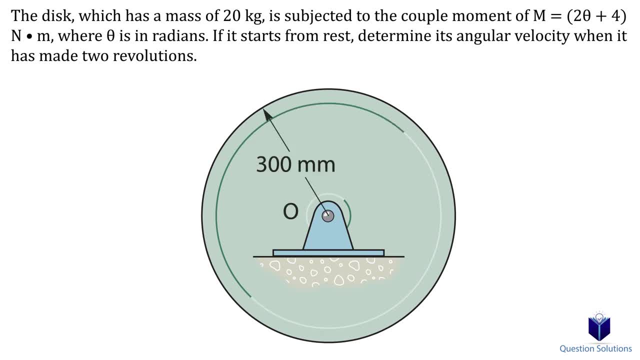 We have a disc and we need to figure out the angular velocity of the disc. We need to figure out the angular velocity of the disc After it goes through two revolutions. let's draw a free body diagram. We have the weight, the reactions at pin O and we have the moment Now for our principle of work and energy equation. 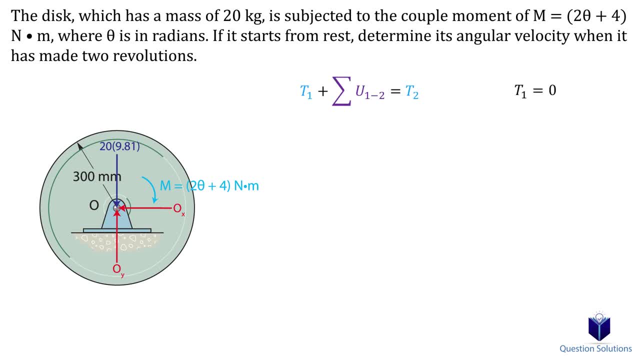 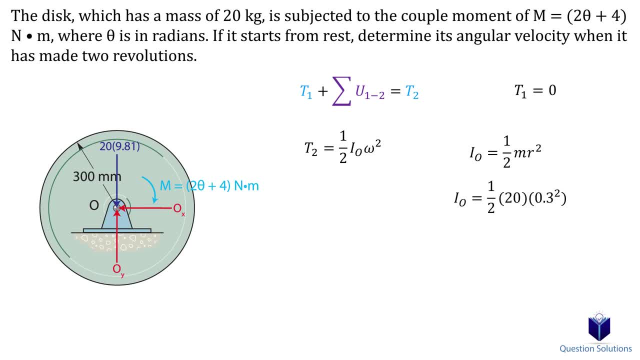 Since point O is the center of this disc, the equation for a uniform moment is 0.0.. The mass is 20 kilograms and the radius is 0.3 meters. Now that we have the mass moment of inertia, we can figure out the final kinetic energy.